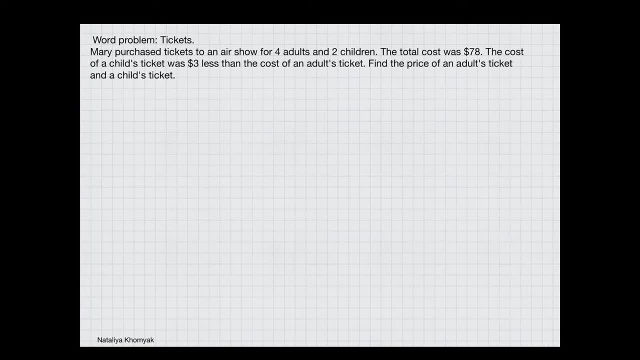 Hi all Here. we have a problem about tickets. So Mary purchased tickets to an air show for four adults and two children. The total cost was $78.. The cost of a child's ticket was $3 less than the cost of an adult's ticket. Find the price of an adult's ticket and a child's ticket. So here we have two categories. We have adult and child's. 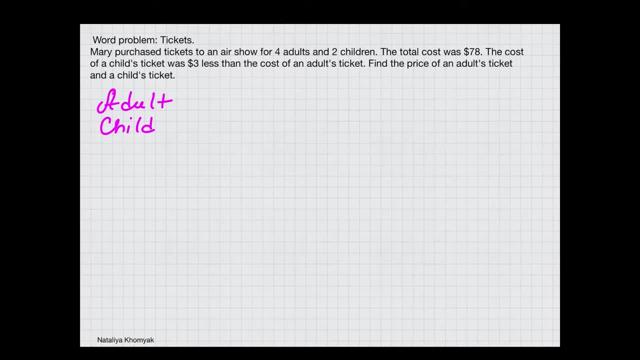 Tickets and child tickets. So let's say adult's tickets are worth X amount of money and the child's ticket is worth Y amount of money, And we know that the total cost was $78.. And we know that she bought four adult's tickets, So four times X. This will give us the price of how much she paid for them. 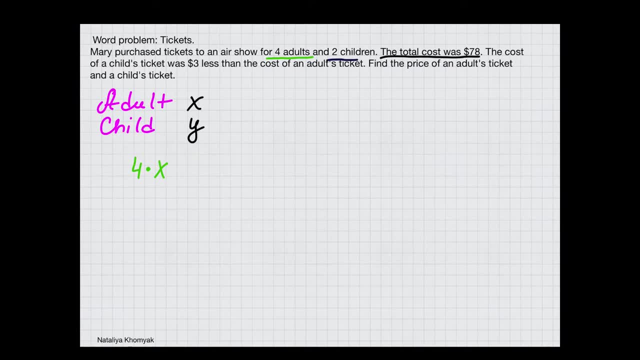 For the adult tickets And we know that she bought two tickets for children. So plus two tickets of how much the child's ticket is worth Y, And all together it was worth $78.. Now we are also told that the price of a child's ticket was $3 less than the cost of the adult's ticket, So the price of the child's ticket was $78. 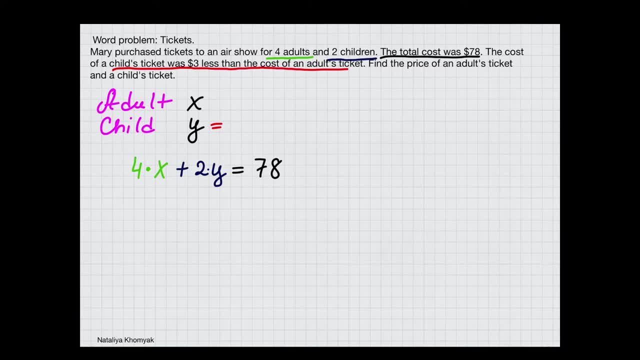 So the price of the child's ticket Y will be equal to if you take the price of how much you would have to pay for adult, which is X, and $3 less would be minus three. So X minus three represents the price of the child's ticket in terms of the adult's ticket. So let's substitute whatever the Y is in this equation in terms of X. 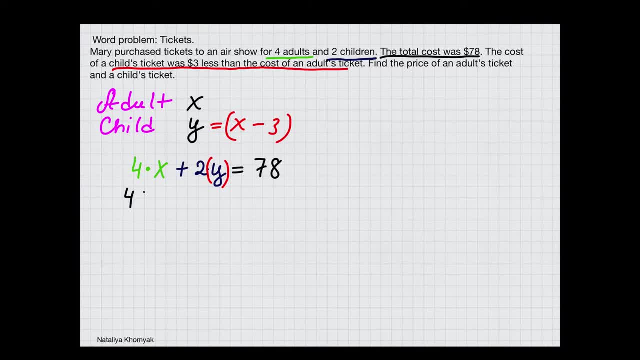 So let's substitute: We have four X plus two times Y equals to 78. And we know that Y is equal to X minus three. So we have four X. Let's distribute the two, So we copy what's inside of the parentheses. We have X minus three And both of these get multiplied by two times, two times two.